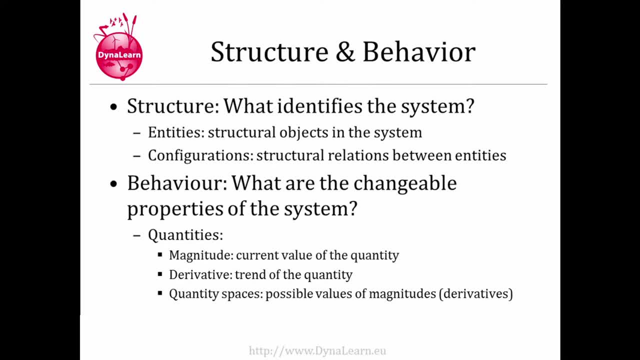 represent the structural relations between entities. Together, these ingredients represent the structure of the system. When modeling the behavior of the system, the question to be answered is: what are the changeable properties of the system? The most important ingredient used to model the behavior of the system are quantities. Quantities consist of a magnitude which represents the 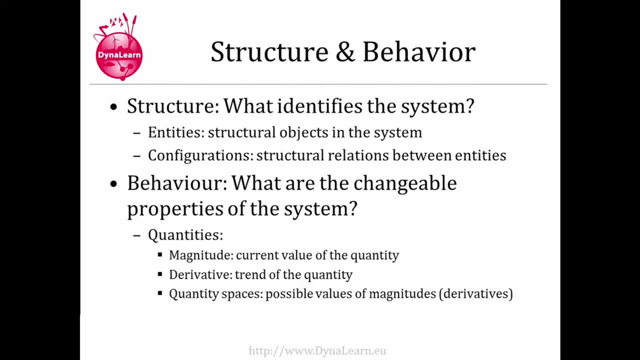 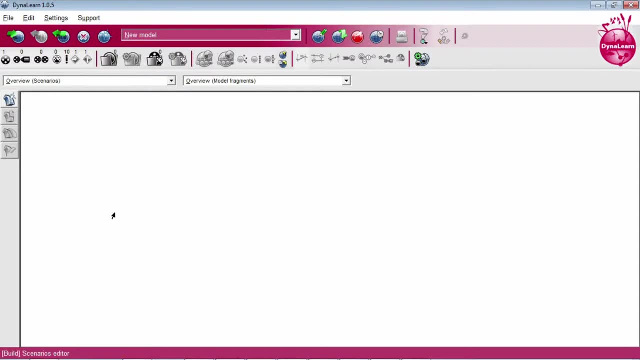 current value of the quantity, a derivative which represents the trend of the quantity, and both the magnitude and the derivative have a quantity space which represents their possible values. So let's see how you would model the structure and behavior in Dynalearn. For this system, the appropriate learning space is learning space 4.. 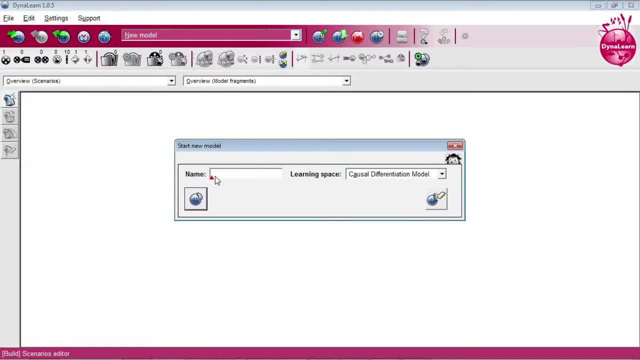 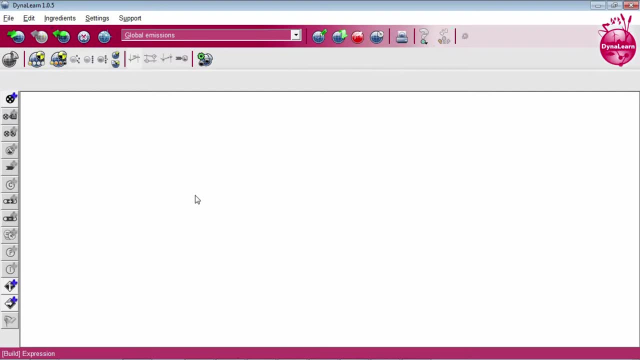 So I will select learning space 4 and I will call this model global emissions. I will start by modeling the structure of the system using entities. The first entity is called global population, The second entity is called atmospheric carbon dioxide And the third is plant population. 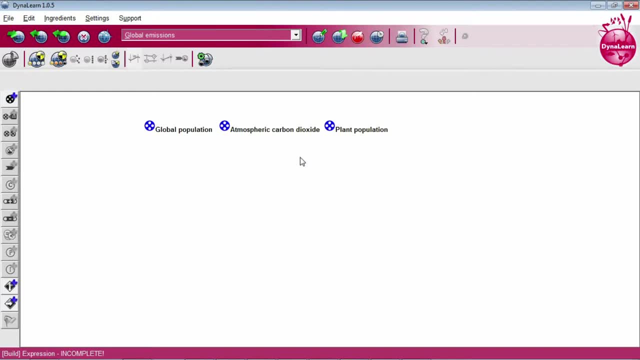 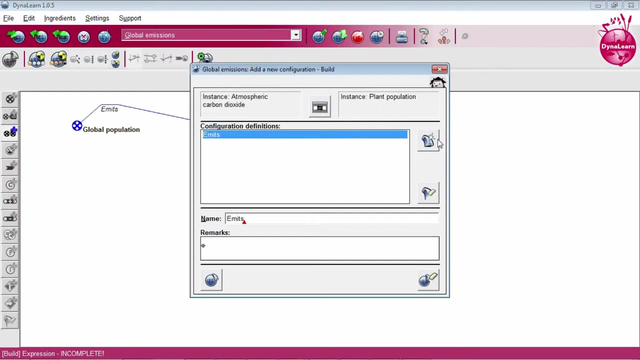 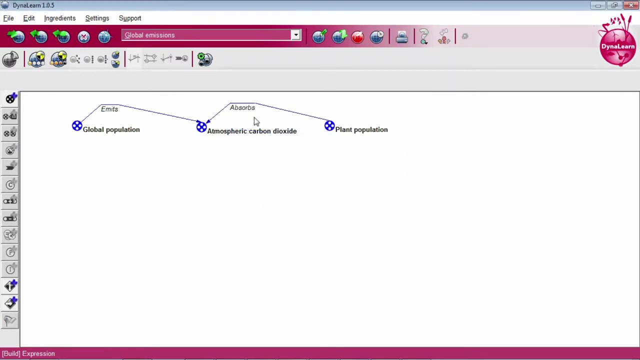 Now I will relate these entities using configurations. The global population and atmospheric carbon dioxide are related by a configuration which is called emits. So this indicates that the global population emits atmospheric carbon dioxide and the plant population absorbs carbon dioxide. So now I've modeled the structure of the system. So now let's start. 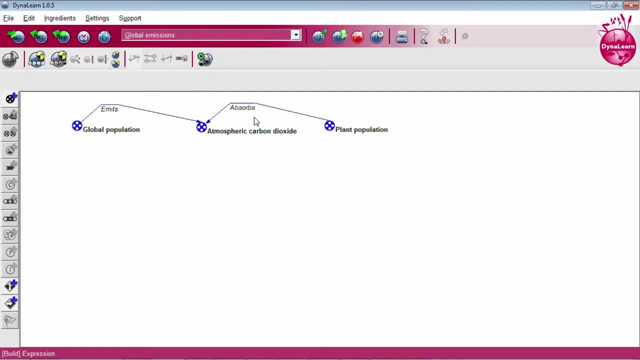 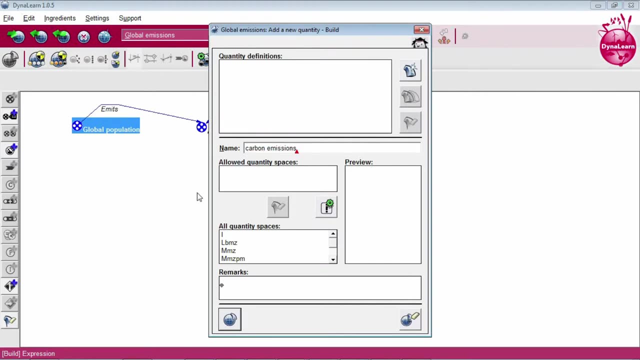 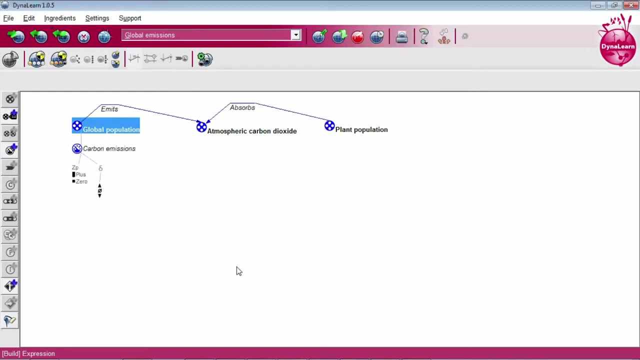 representing the behavioral aspects of the system using quantities. The global population has a quantity which is called carbon emissions. I will indicate that this quantity can only have the values zero or some positive value. The atmospheric carbon dioxide has a quantity which is called amount. 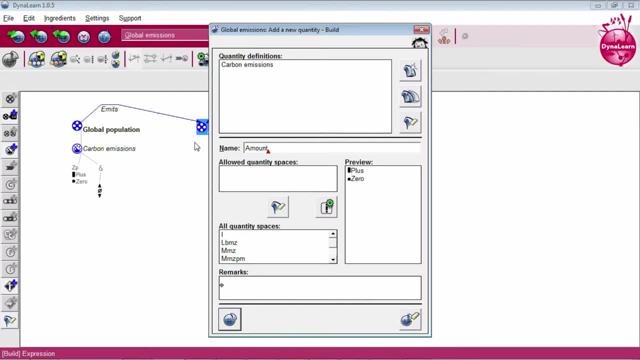 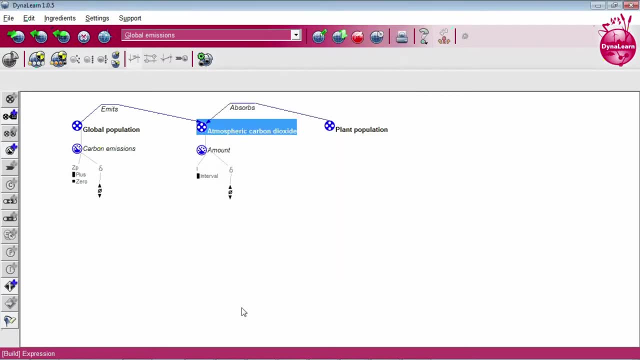 And this quantity represents the amount of atmospheric carbon dioxide. And since I'm only interested in the trend of this quantity, I will only give it one possible value. And finally, the entity plant population has a quantity- photosynthesis, which can also only be zero or have some positive value. 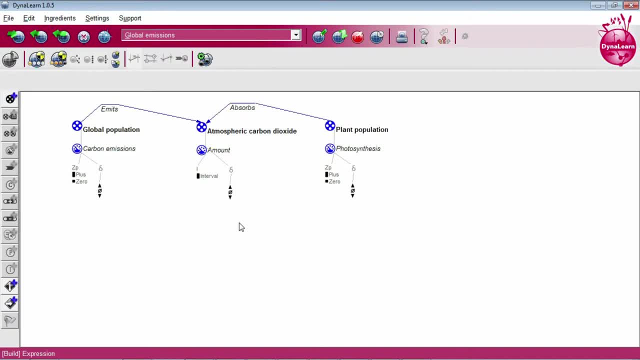 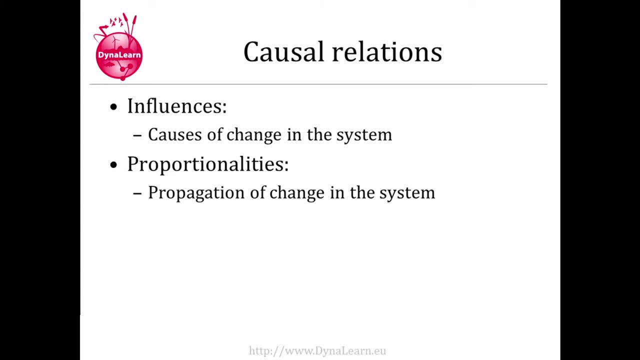 So my model until now represents the structure and part of the behavior of the system. We will now move to the next part of the model, the causal relations. Dynalurn provides two types of causal relations. First, influences represent the causes of change within a system. Second, proportionalities propagate the 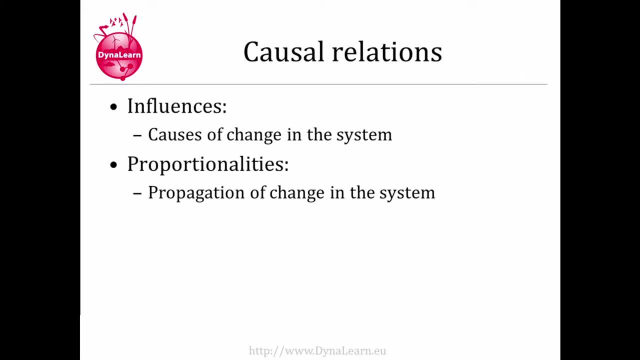 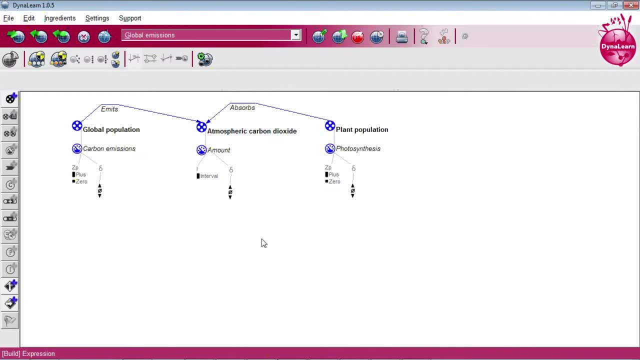 change that is caused by the changes in the system that is caused by these influences. So let's add some of these causal relations to our model. In this system there are two important causal relations and they are both causes of change. First, the carbon emissions cause the amount of atmospheric carbon dioxide to increase. 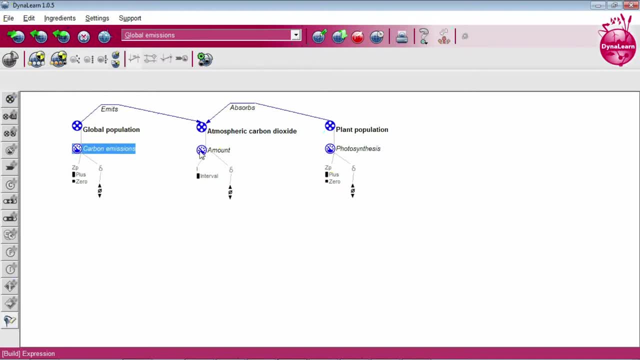 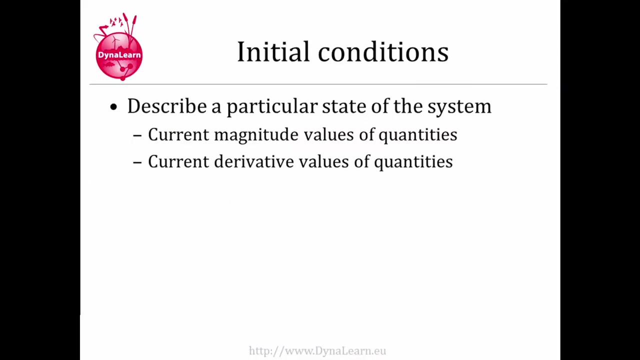 So there is a positive influence between these two quantities. Second, photosynthesis decreases the amount of atmospheric carbon dioxide through absorption. Therefore there's a negative influence between photosynthesis and amounts. So now we've modeled the causal relations within the system. Now we will move to the initial conditions. 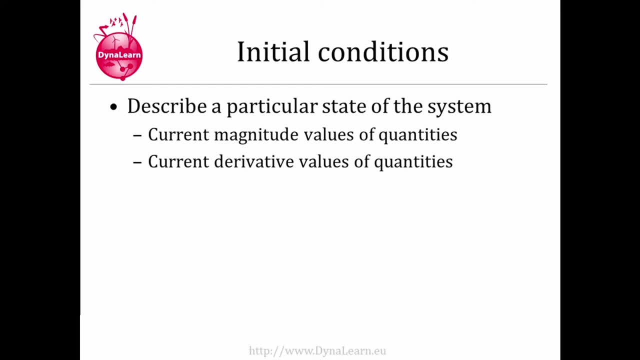 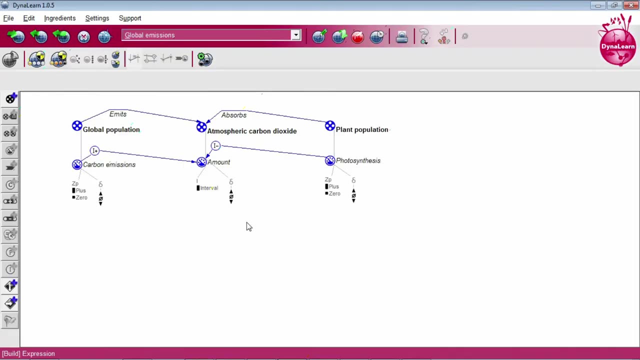 The initial conditions are a set of values that describe a particular state within the system. This state description will be the basis for the simulation. These values include the current magnitude values of quantities and the current derivative values of quantities. We are interested in the trend of the amount of atmospheric carbon dioxide. 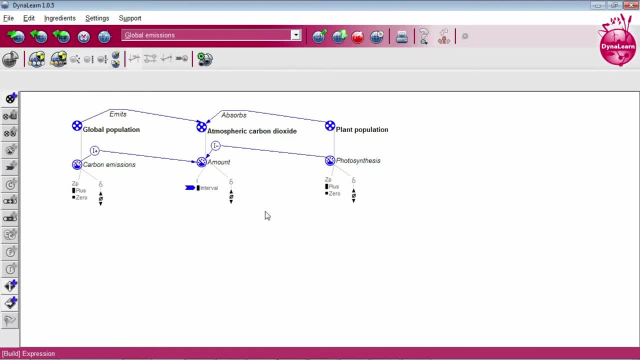 so we will indicate that it has some value, But we will leave the derivative open, as this describes the trend of the quantity and we want to derive this trend in terms of the amount of atmospheric carbon dioxide. For the carbon emissions, we will indicate that it is above zero and that it is currently steady. 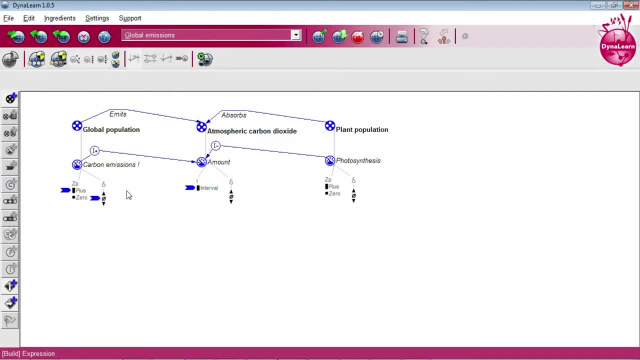 This corresponds to the typical answer that was given to the exercise, which was that, in order for the amount of atmospheric carbon dioxide to stabilize, the carbon emissions have to stabilize in the year 2100.. And finally, photosynthesis. This represents the net removal in the exercise. 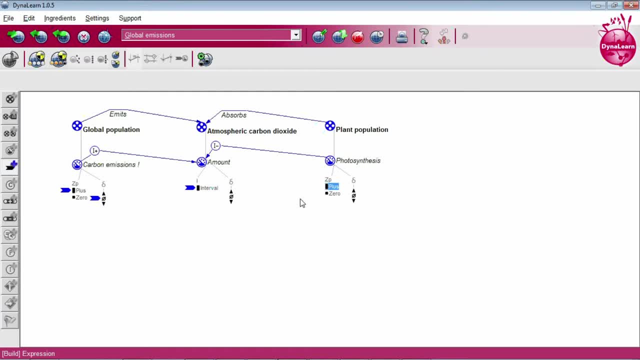 In the exercise the net removal is above zero and does not change. so we will do the same for photosynthesis. So now we have completed the initial conditions of the system and are now able to run a simulation. The typical answer to the exercise indicated that if the carbon emissions stabilize, 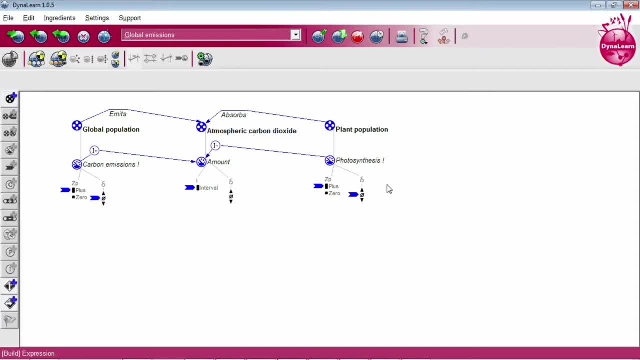 the atmospheric carbon dioxide will also stabilize. We will now run a simulation to check whether this answer is correct. The simulation shows that there are three states, which means that the system can behave in three distinct ways. This is not what we expected. We expected only one state in which atmospheric carbon dioxide has become stable. 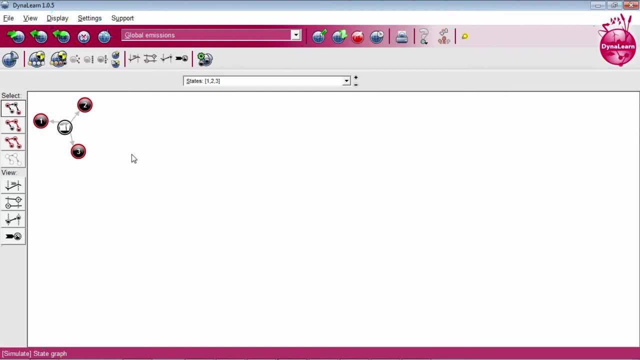 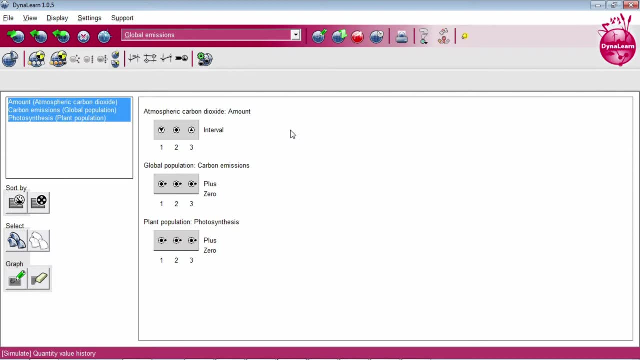 We can look at the values of the quantities in each of these states to figure out what has happened Here. we can see that atmospheric carbon dioxide can either decrease, be stable or increase, even though the carbon emissions are stable. This means that the typical answer that is given in the exercise is actually incorrect. 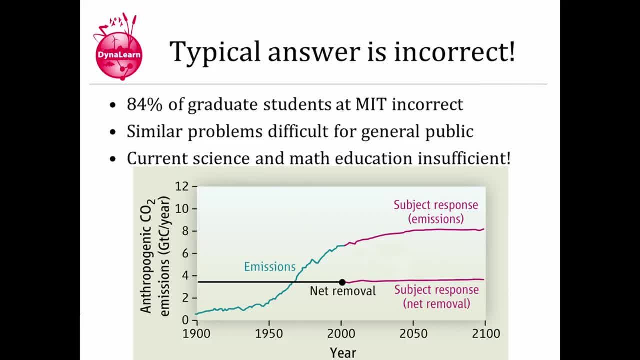 And in a study performed at MIT, the researchers found that 84% of their graduate students gave an incorrect answer to this exercise. The students were highly trained in science and mathematics and had backgrounds that included physics, mathematics and economics, And there is a large body of research that indicates that the general public 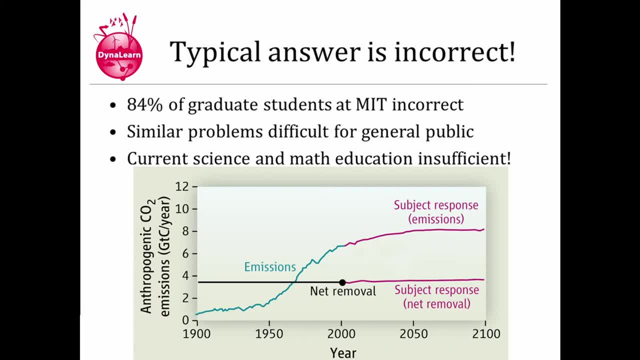 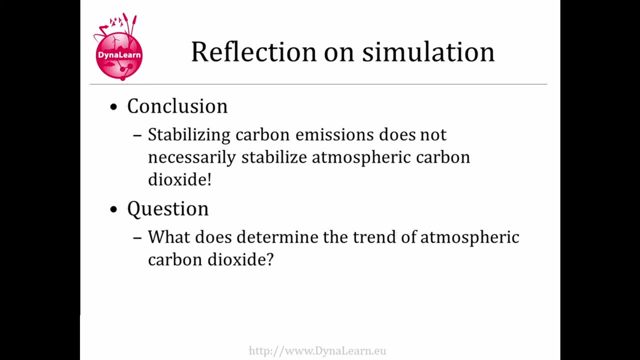 struggles with similar problems. So the conclusion here is that current science and math education insufficiently prepares learners to think about dynamic systems. So does conceptual physics change? conceptual modeling and simulation provide an answer. Reflecting on the simulation results, we should draw one conclusion: Stabilizing carbon emissions does not necessarily stabilize. 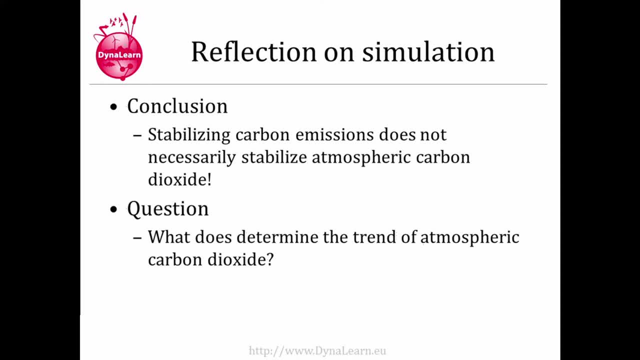 atmospheric carbon dioxide. We saw in the simulation results that the atmospheric carbon dioxide could either increase, decrease or be stable. So the question that we should ask is: what does determine the trend of atmospheric carbon dioxide? So let's alter the model to see if we can figure that out. 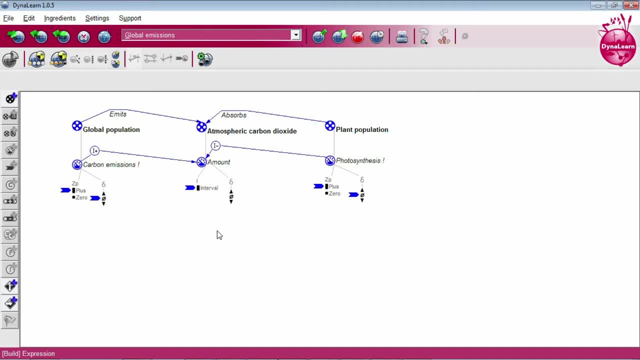 We know now that carbon emissions being stable does not cause the atmospheric carbon dioxide to be stable. So what does determine the trend of atmospheric carbon dioxide? We can think of the atmosphere as a bathtub and the carbon emissions as an inflow from a faucet. 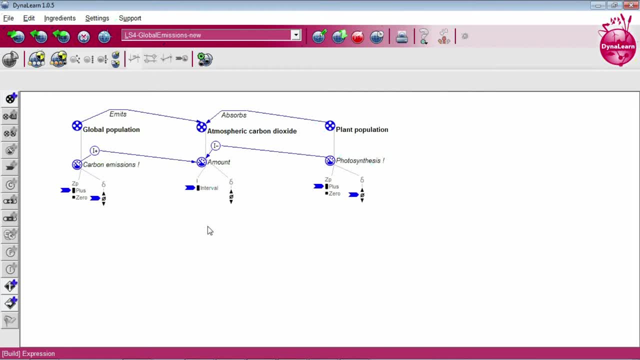 and the photosynthesis as an outflow from a drain. So probably what is important is the relative strengths of the inflow and the outflow, in this case the carbon emissions and the photosynthesis. To check this out, we should first look at the atmospheric carbon dioxide.